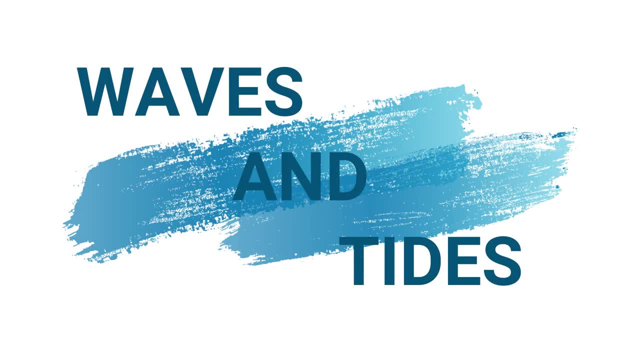 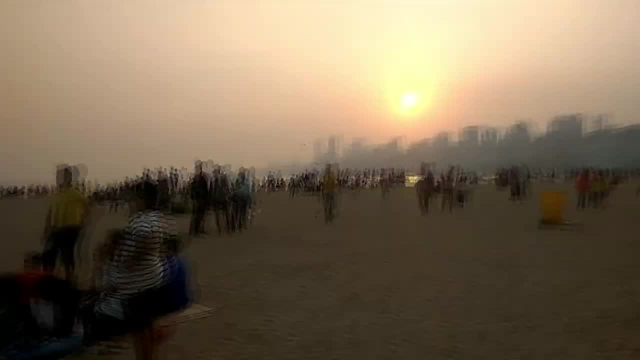 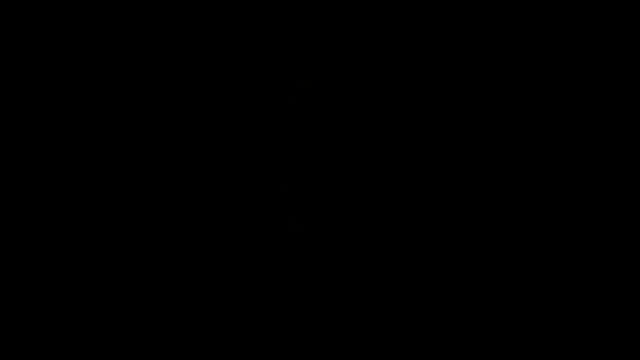 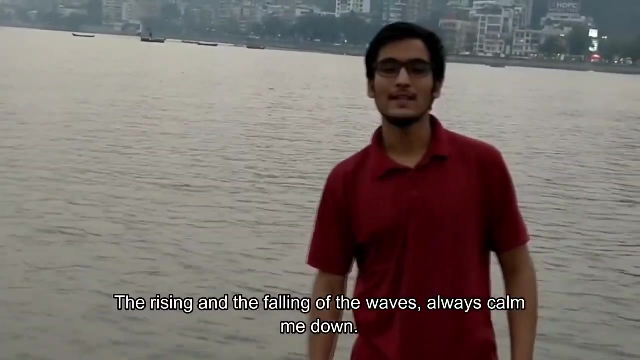 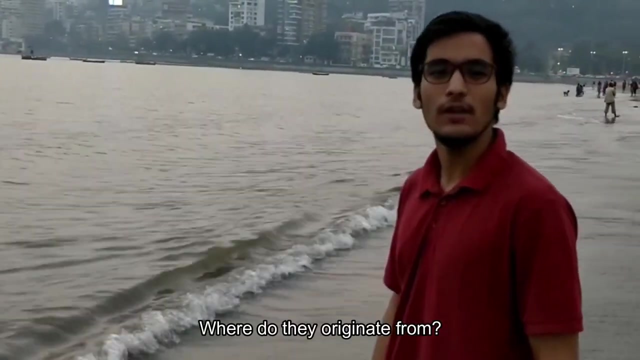 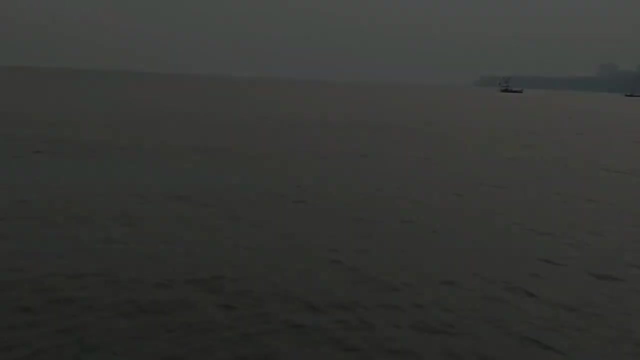 I always feel nice when I come to this sea. The rising and the falling of the waves always calm me down. But have you ever wondered why these waves form? Where do they originate from? Let's look into the physics of it. A wave, in simple physical terms, is an oscillation. 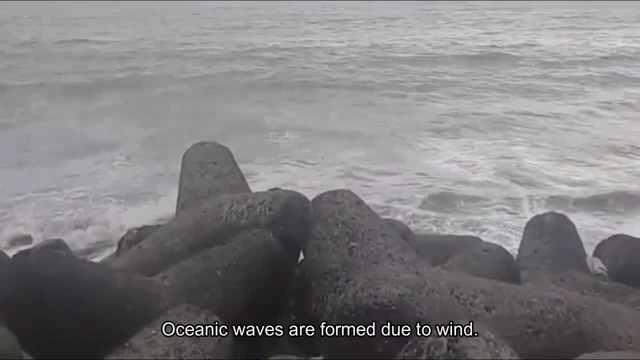 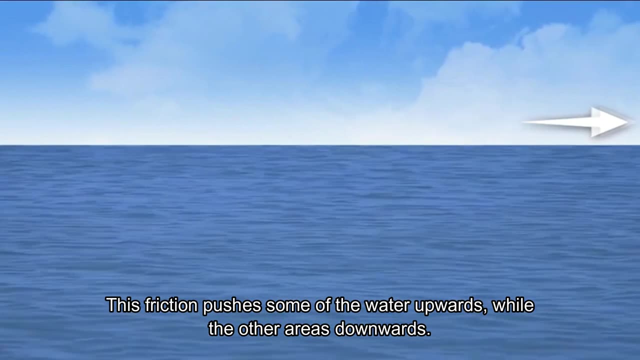 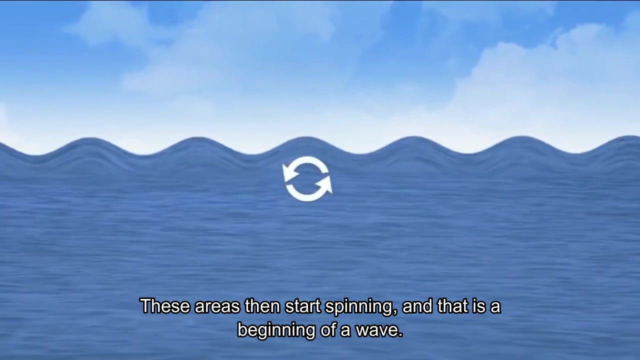 with a transfer of energy. Oceanic waves are formed due to wind. When wind blows over the surface of the water, it creates friction. This friction pushes some of the water upwards, while the other areas downwards. These areas then start spinning, And that is the beginning. 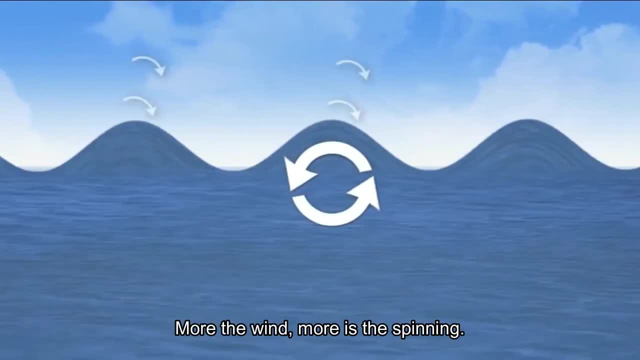 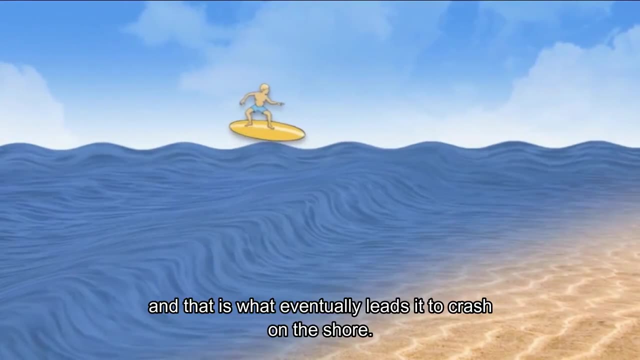 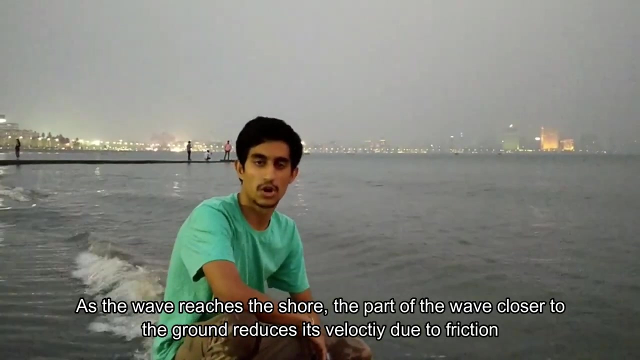 of a wave. More the wind, more is the spinning. As we go closer to the shore, the spinning causes the water to bob up and down And that is what eventually leads it to crash on the shore. Why do these waves break? As a wave enters the shore, the part of the wave blows. 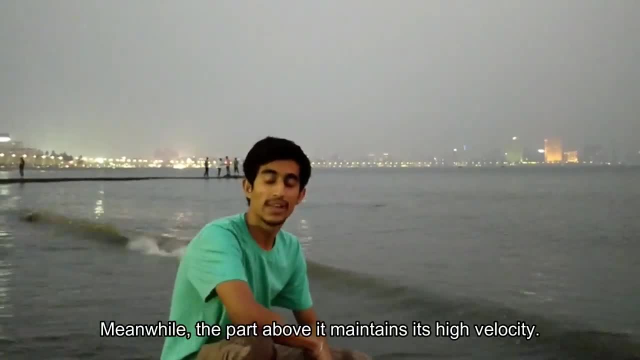 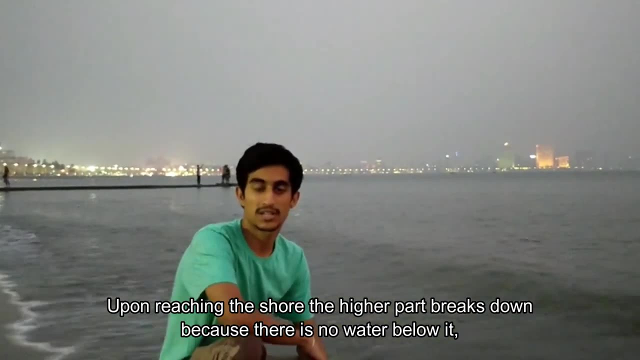 to the ground and reduces its velocity due to friction. Meanwhile, the part above it maintains its high velocity. Upon reaching the shore, the higher part breaks down because there is no water below it. This results in the wave breaking down. Tsunami is a word. 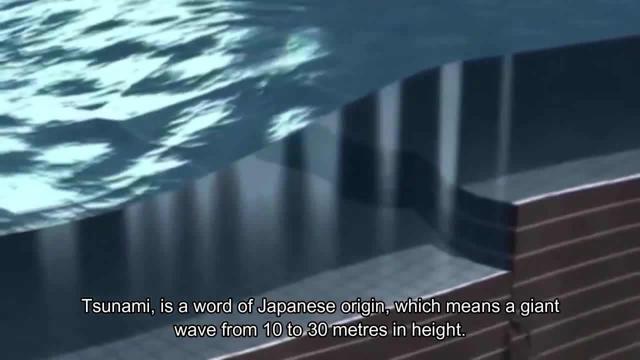 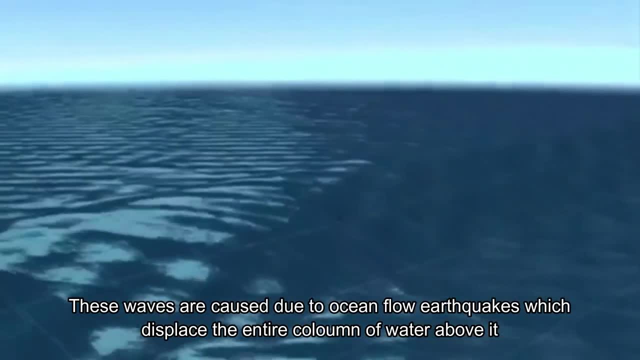 of Japanese origin, which means a giant wave from 10 to 30 meters in height. These waves are caused due to ocean floor earthquakes, which displace the entire column of water above it, which then ripples outwards, As opposed to wind waves, which displace water till only. 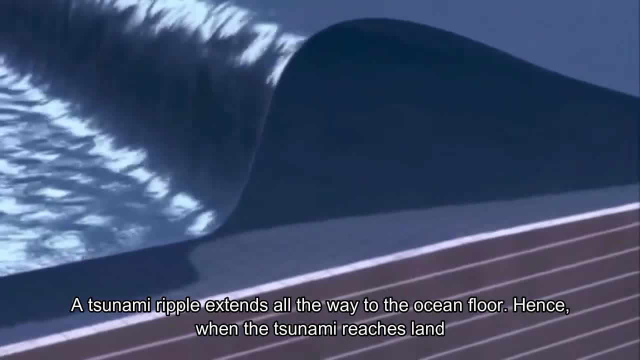 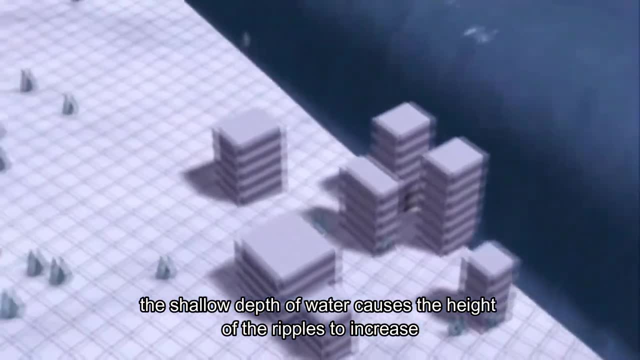 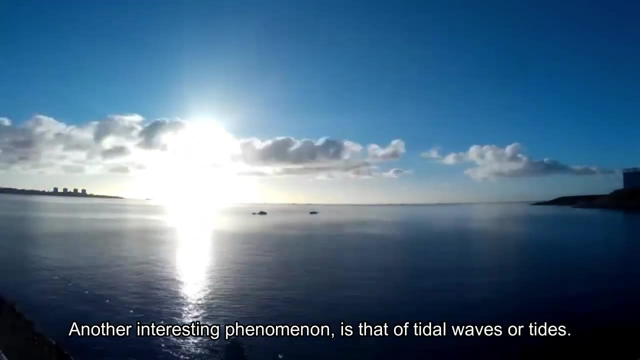 below the surface, a tsunami ripple extends all the way to the ocean floor. Hence, when the tsunami reaches land, the shallow depth of water causes the height of the ripples to increase, creating the destructive wave that is so famous. Another interesting phenomenon is that of tidal waves or tides. It is the cyclic rising and falling of the earth's ocean. 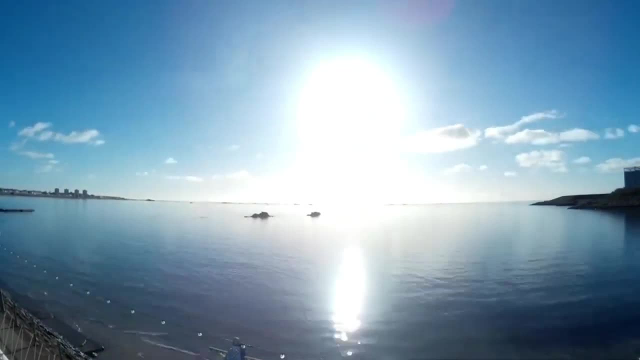 surface, which is caused by the tidal forces of the moon and sun. Basically, what we observe over a day are changes in the depth of the waves. These changes are called tidal waves. The tidal waves are the waves that are formed by the tidal forces of the moon and sun. Basically,